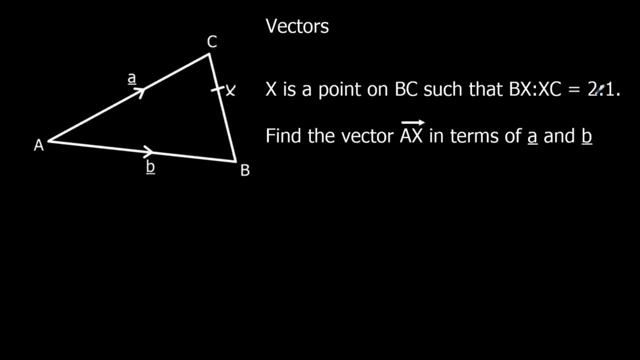 this is x here. b to x is two parts and x to c is another one part. So this is two parts. This is one one part. So we can say that B to X is two out of three, two thirds of the journey, and X to C is: 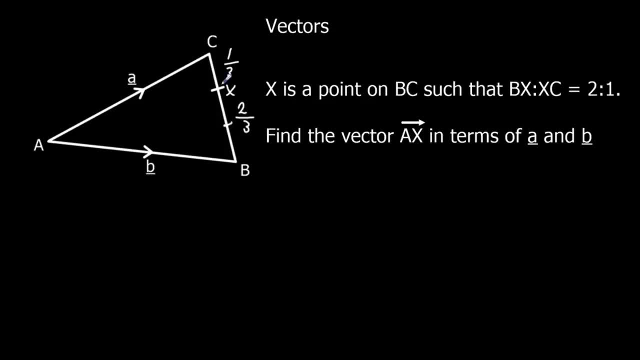 one third. So B to X is two thirds of the whole line, B to C and X to C is one third of it. Okay, so we need to go from A to X. So if there was a part A to this question, the part A would: 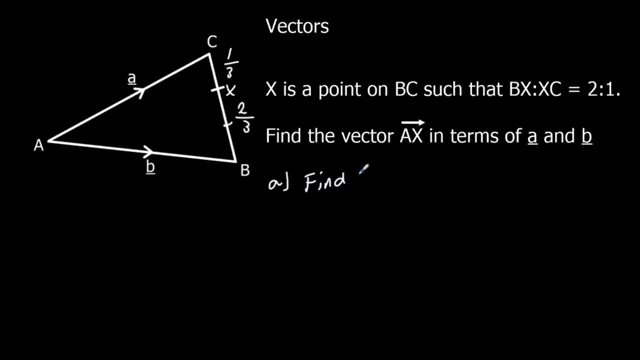 say find B to C in terms of A and B, So let's find B to C first. So from here to here, we can't go up here, it hasn't got a name, So we're going to go B to A, which is backwards along the B. So it's. 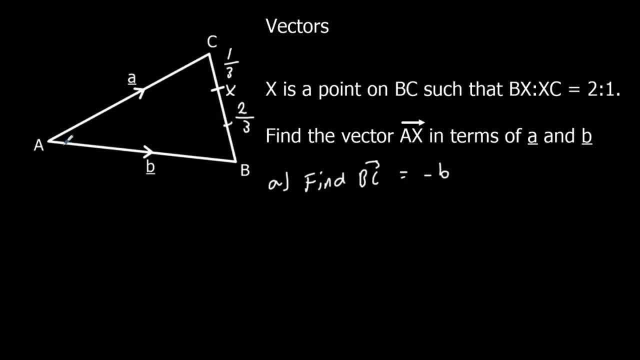 going to be minus B backwards along the B, And then we're going to go forwards up the A, so minus B plus A, So that's B to C. So now I'm going to go A to X, So A to X is going to be A to B, and do A to B first, And then I'm 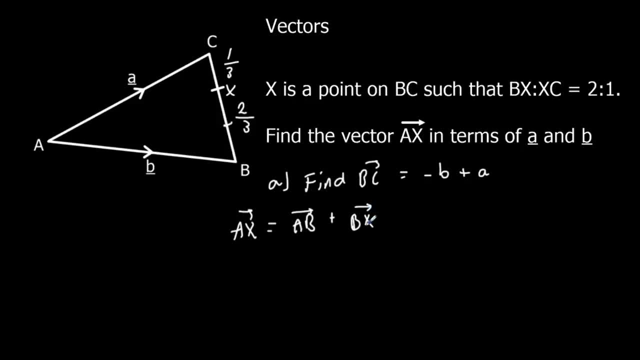 going to go from B to X. So A to B, that's our B, And then B to X. that's two thirds of this journey. So two thirds of B to C. So two thirds of B to C. And then we need to simplify this by expanding the bracket. So we're going to have B and then 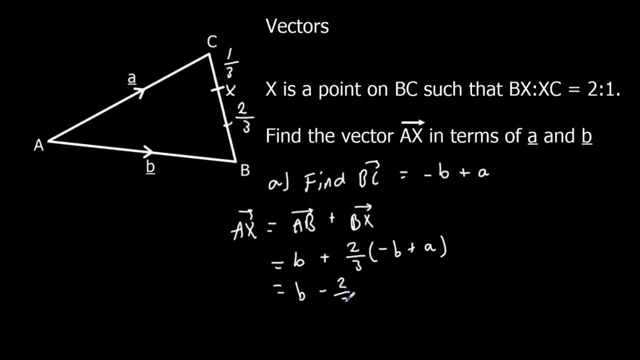 two thirds times minus B is minus two thirds B, And two thirds times A is two thirds A. So it's no different. saying two times A is two A, it's two thirds. Two thirds times A is two thirds A And I've got a whole take away two thirds of the B's, So one whole take. 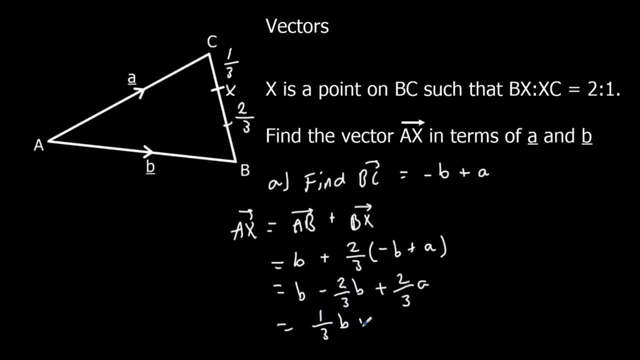 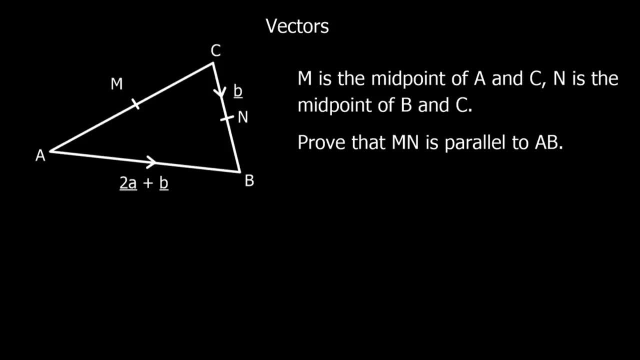 away two thirds of the B's, so one whole take away two thirds of the B's, So one whole take away two thirds is one third. So I've got one third B and two thirds A, And that's the answer. Okay, M is the midpoint of A to C, So that's here. 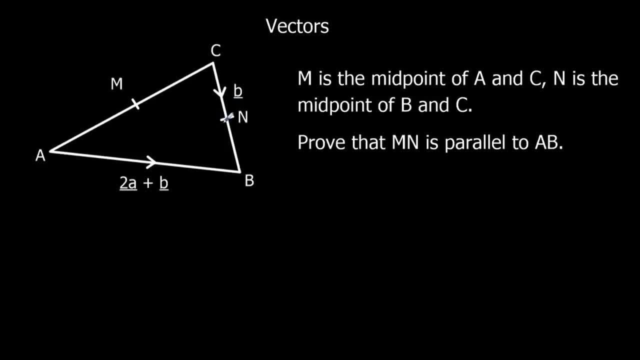 And N is the midpoint of B and C. So that's in the middle here. Prove that M- N is parallel to A- B. So to go from M to N again, if there was a part A, it will be find A to C. 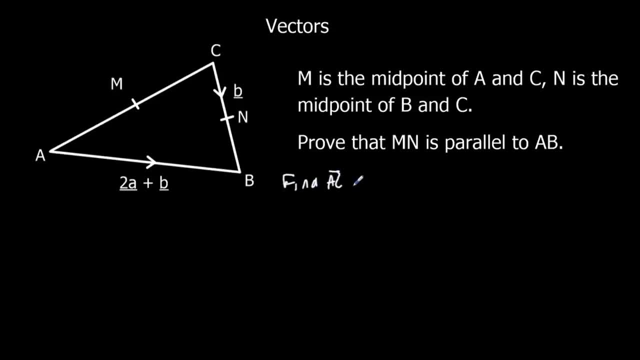 So find A to C in terms of A and B. So A to C, I'm going to go A to B, and then I'm going to go from B to C. So A to B, this time it's two A plus B. 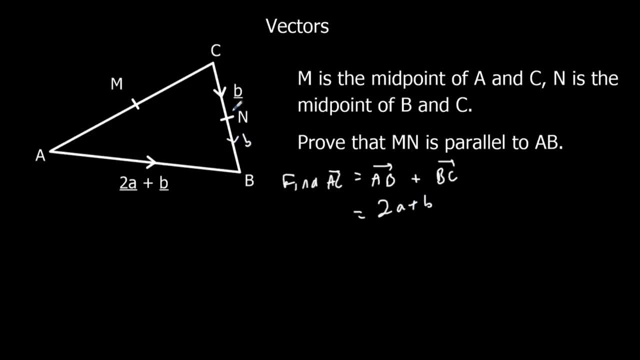 And B to C. I think that should be there. So that's halfway is called a B, so the other half's also called a B. So So B to C is minus B minus B, which is minus two Bs. So A to C is two A minus a B. 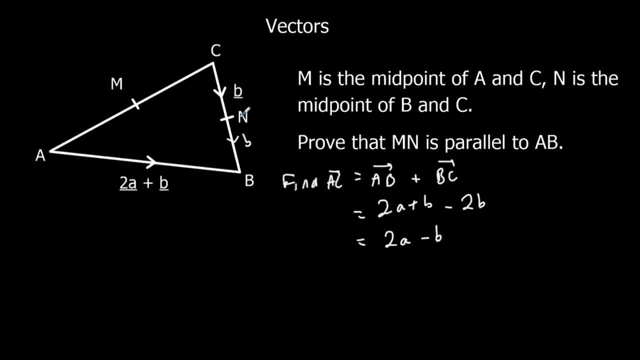 So that's A to C. We need to go M to N. So we're going to find M to N. We already know A to B and then we'll see what parallel means after. So let's go from M to N. 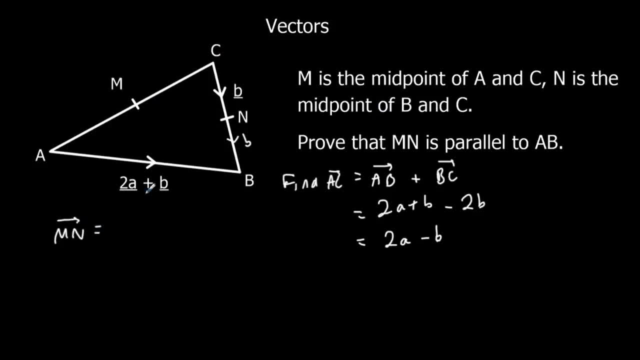 So M to N is going to be M to C and then C to N. So M to C is half of A to C. So half of A to C and then plus a B. So we expand the bracket half times two, that'll be one. 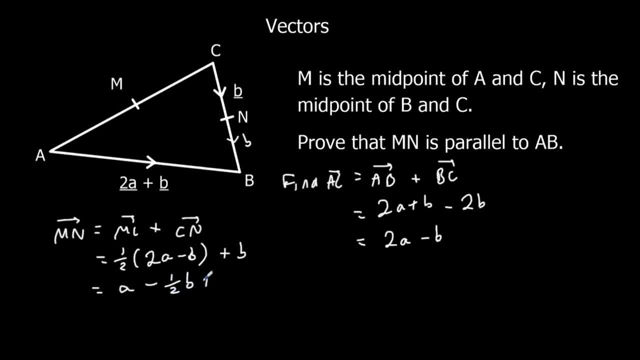 Half times two Half times two Half times minus B is minus a half B, Minus a half B. plus a whole B is plus a half Plus a half B. Right, so now we've got M to N, This is M to N, and we've got A to B. 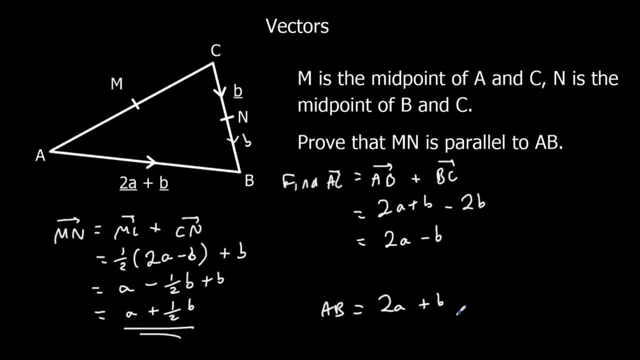 A to B is two A plus B. How do we prove they're parallel? So, to be parallel, one has to be a multiple of the other one. So is one a multiple? Is one a multiple of the other one? Well, yes, it is. 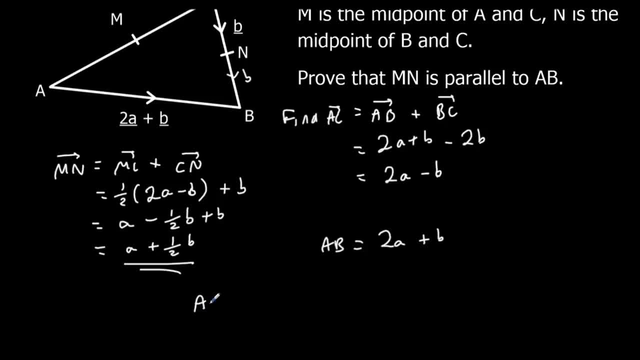 So A to B is equal to two lots of MN. So because it's a multiple, because MN is a multiple of AB or AB is a multiple of MN, but because one is a number times the other one, that means they're parallel. 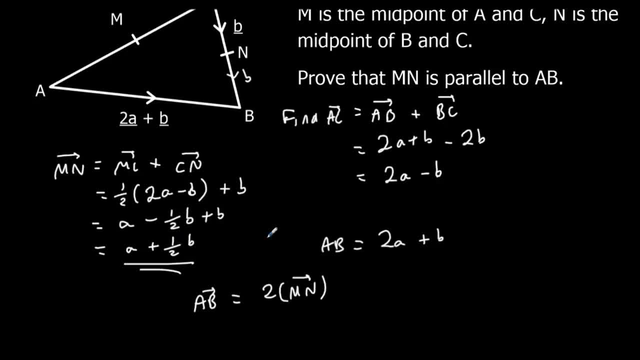 They're going in the same direction. If I went along two MNs, I've gone along an AB, So they're going in the same direction. AB is a multiple of MN. Therefore MN is parallel to AB. Okay, here's another question. 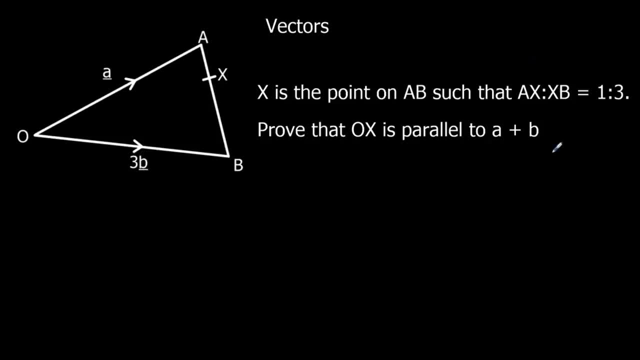 So X is the point on AB, So that's that. So AX is one part, So it's one part, And XB is three parts, So three parts down there, So it's in four parts in total. 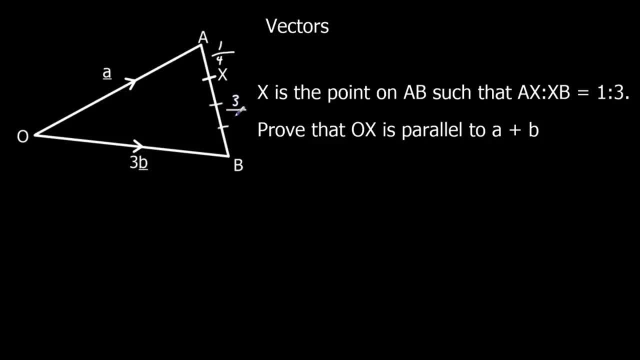 So this is one quarter And this bit here, the big bit, is three quarters. And then we need to go O to X. We need to prove it's parallel, So a multiple of A plus B, So O to X is going to be there. 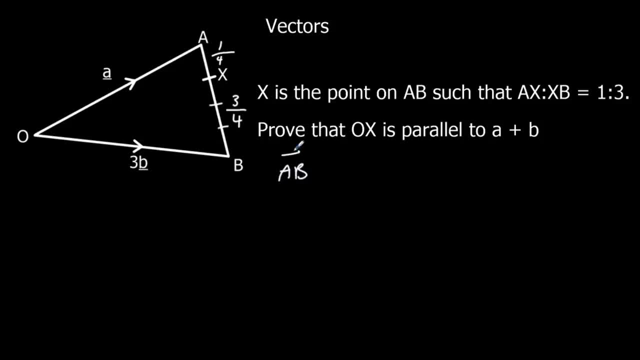 So to do that, firstly we need to find A. So let's go from A to B first. So we're going to go minus an A down to O. So minus an A And then plus 3B. 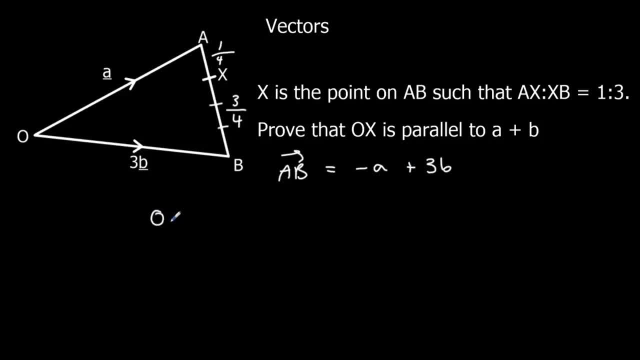 That's A to B, And then, if I want to go O to X, I'm going to go up O to A And then I'm going to go from A to X, which is a quarter of AB. So O to A is an A plus a quarter of AB, minus A plus 3B. 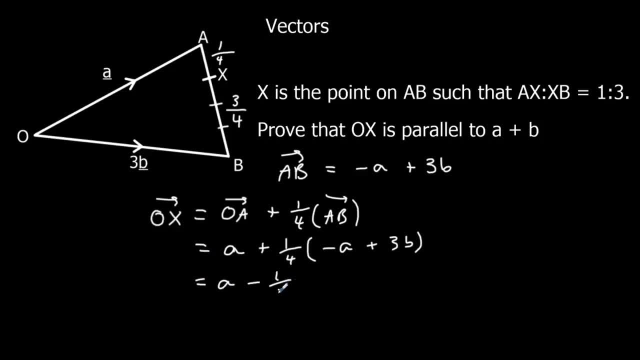 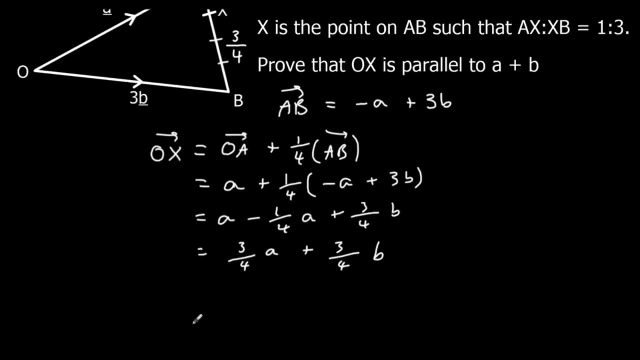 Expand the bracket So it's minus a quarter A plus three quarters B, One whole. take away a quarter, that's three quarters, That's three quarters B. So we can see that that's parallel, Parallel to AB. AB is three quarters. 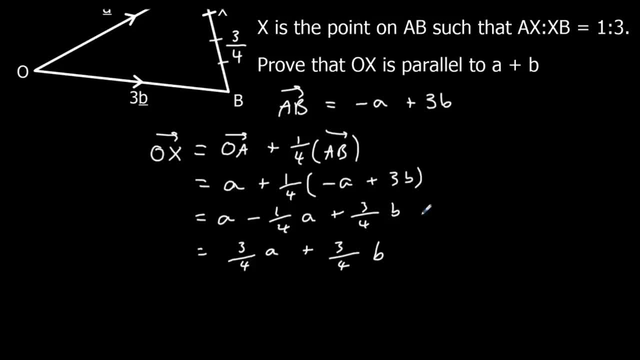 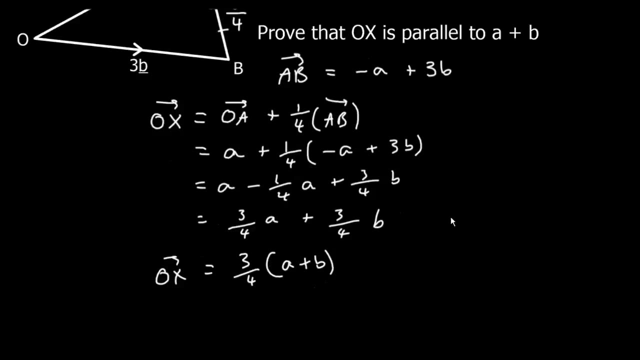 I mean yep, A plus B is. this is O to X is three quarters of A plus B. So O to X is three quarters of A plus B. Therefore O to X is parallel. Parallel to AB, Class B. 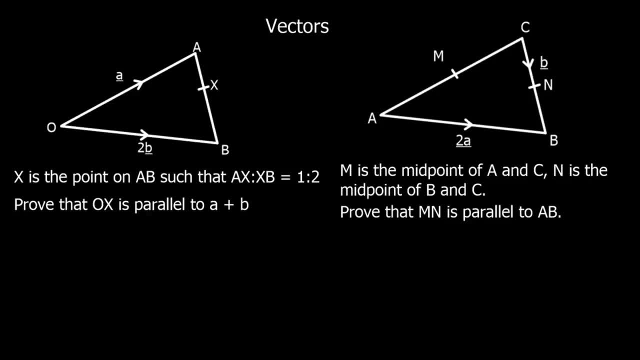 Okay, so you can give these two questions a go. So see if you can answer two questions. Pause the video and give them a go. Okay, so this first one over here. So AX to XB is one part to two parts. 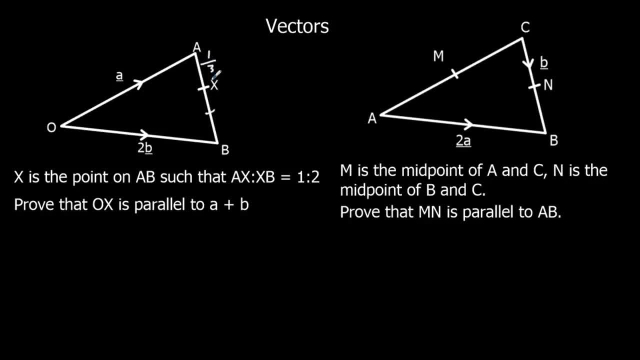 So that means AX is one-third of the total and X to B is two-thirds. We go from O to X. So firstly we need to know A to B. A to B is minus an A and then plus 2B. 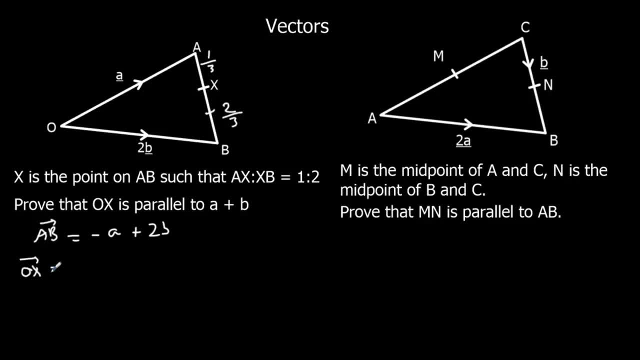 And O to X. that would be O to A And then one-third of A to B. So O to A is an A and then we've got one-third of minus A plus 2B. Expanding the bracket gives us minus a third A plus two-thirds B. 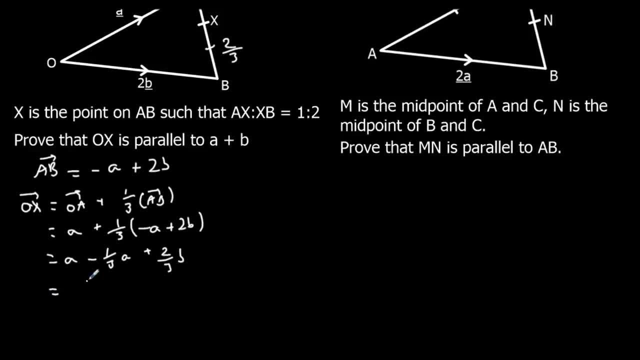 And a whole takeaway of thirds is two-thirds. so we've got two-thirds A plus two-thirds B. So O to X is two-thirds of A plus B. Therefore they're parallel because it's a multiple. It's a multiple of A plus B, It's two-thirds of it, so it's parallel to it. 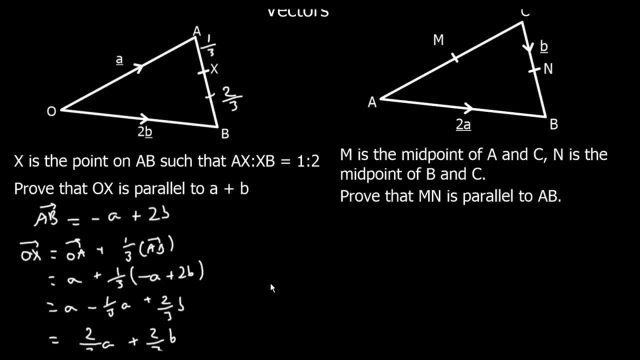 M is the midpoint of A and C. M is the midpoint of A and C. here, N is the midpoint of B and C. Prove that MN. MN is parallel to AB. So we need to go from M to N, So we need to know AC first. 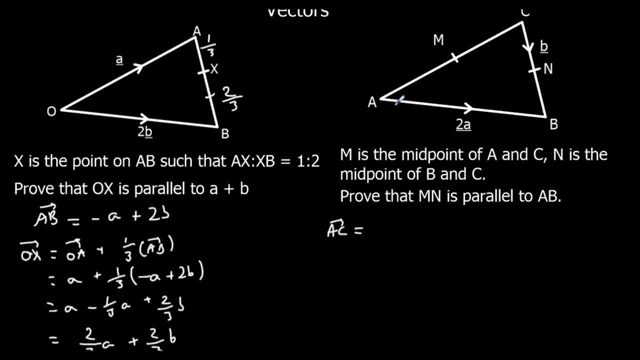 So let's find AC first. It's 2A minus 2B, So there's a B there and a B there, 2A minus 2B. So we need to M to N. M to N is half of A to C. 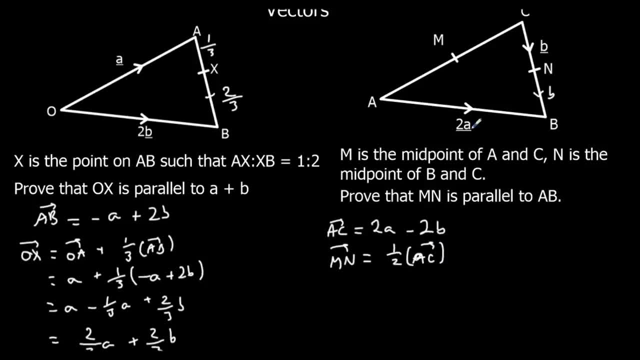 Half of A to C And then plus C to N, which is a B plus C to N. So half of A to C, half of 2A minus 2B plus a B. Half of 2 is just 1, so B A minus B plus B, and that gives me A. 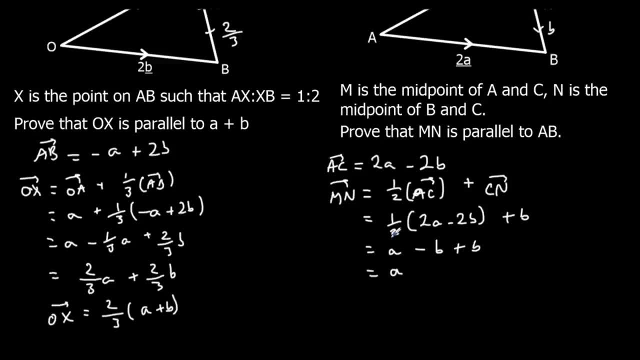 So M to N is just an A. So is it parallel? Yes it is, Because M to N is half of A to B. So therefore, because it's a multiple, it's parallel. So therefore they are parallel. So two lines are parallel if one's a multiple of the other. So it's a parallel if one's a multiple.